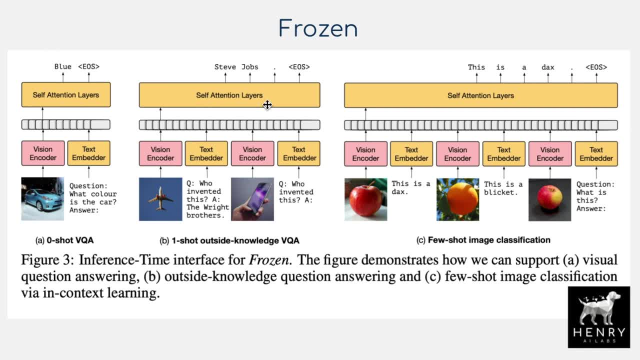 into the details of how exactly this works, but the high-level overview is that you freeze the parameters of the pre-trained language model, hence the name Frozen. You take images, you encode them with a vision encoder, map them to- in this case, two tokens, so the 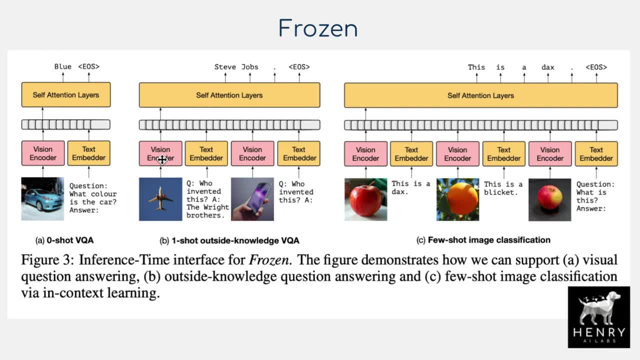 vision language model and then you add vision embeddings to that input sequence. The vision encoder has that vector representation and then funnels it into two tokens to append to the representation. and then this is for each of the input images. You could have alternating. 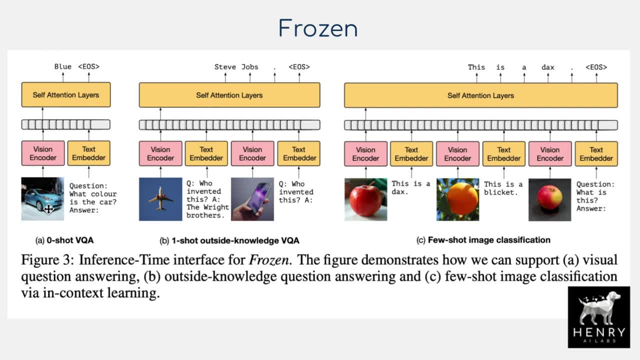 images that's shown in this picture and this picture, or you could just have something like this where you have a car, what color is the car? and these kinds of questions. So these are the kinds of tasks- visual question answering and this few-shot image classification- and then we'll 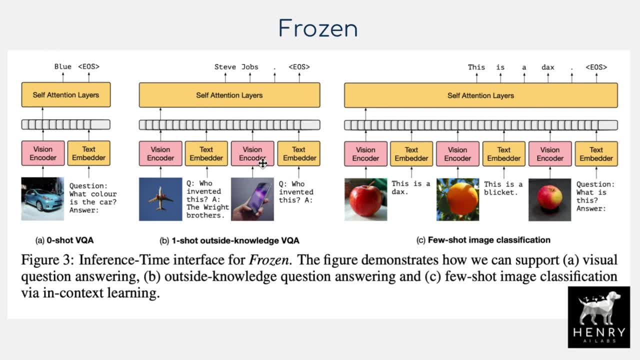 dive more into the details of how they train this vision, encoder the conceptual captions, data set that they use, and then, more particularly, the evaluation of few-shot learning, comparing the image classification, and then we'll dive more into the details of how they train this. 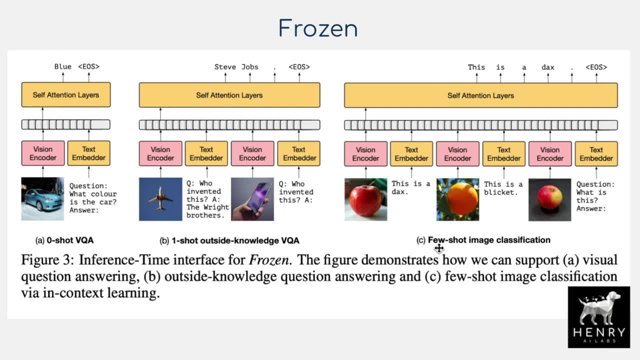 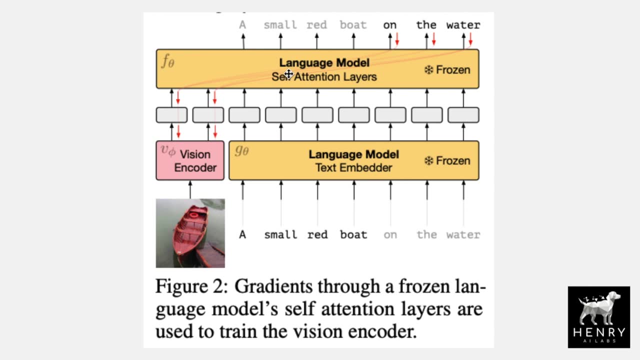 vision encoder. So here's how the Frozen model is trained: You freeze the parameters of the language model, meaning that they're not updated during the training, but the gradients get back-propagated into the vision encoder. So the vision encoder takes in the image and then maps. 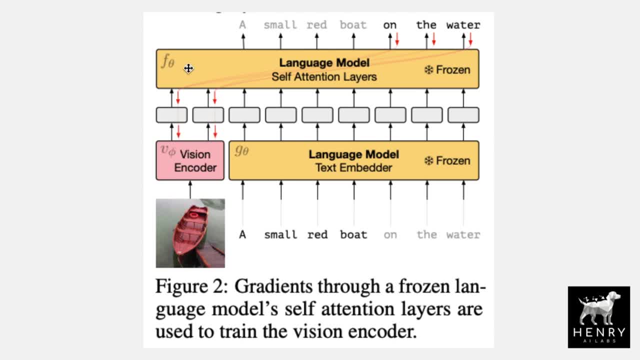 it into the vector representation but then goes into these two tokens and then you have a token slots to the language model. So I'm not sure exactly how this works. It has something to do with, say, each of the dimensionality of the token embeddings as each of the embeddings of a token 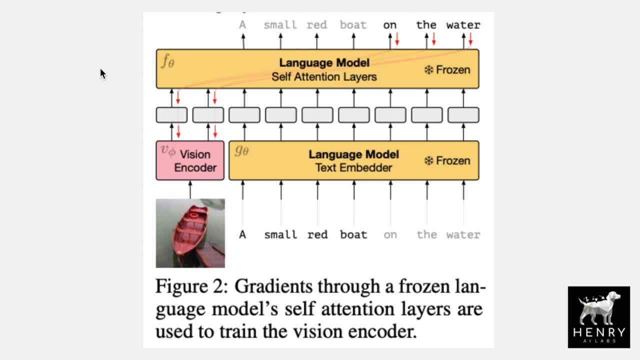 in a language model's vocabulary, say, has a dimension of 512 as a typical vector length. So I put two 512-dimensional vectors to represent this image of a red boat. So you have the data set as conceptual captions. So this is three million image-text pairs of image captioning. So 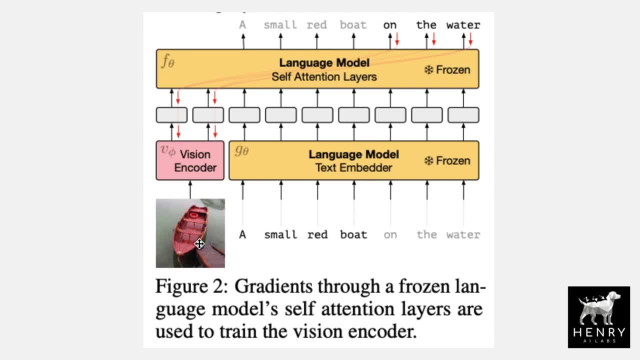 the task is to write the natural language description. The core of this is to write the text. The text corresponds with the image, like this one: a small red boat on the water. And then one of the details of this is that they are hyper-named, meaning that there aren't any named. 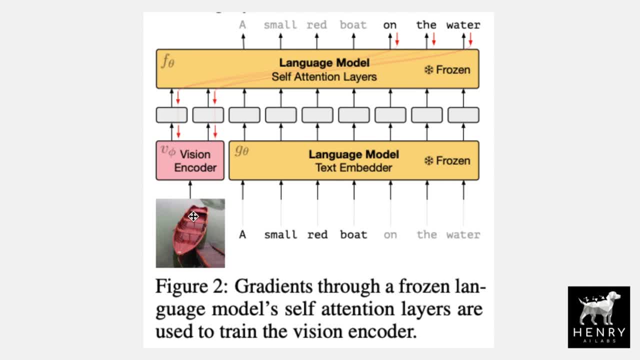 entities in the data set. So if there was a celebrity picture, they would change that into man or woman, And if there's something like a branded anything, they would change that into a bottle or whatever the branded thing was. So there are no named entities in this conceptual. 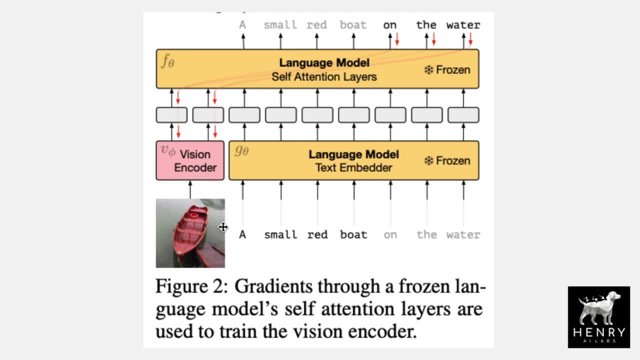 captions, data set, which is why, when they later on test this external knowledge retrieval thing, it's even more interesting Because it has to be getting this from the frozen language model. It can't possibly have learned it in the pre-training task. And then the last detail that might be interesting is that they can't 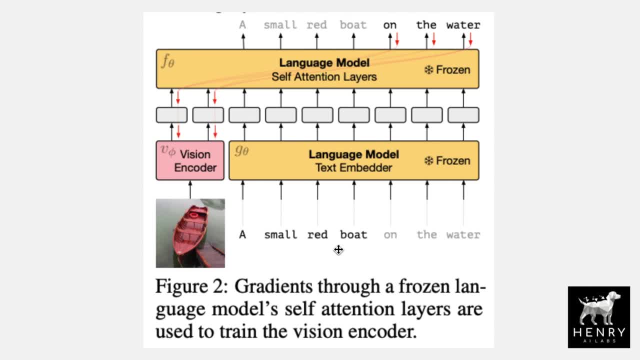 fine-tune the language model, they say, because there isn't enough of this paired data. They have three million pairs. So actually fine-tuning the language model would decrease the performance of the language model compared to the massive amount of data it was pre-trained with through language. 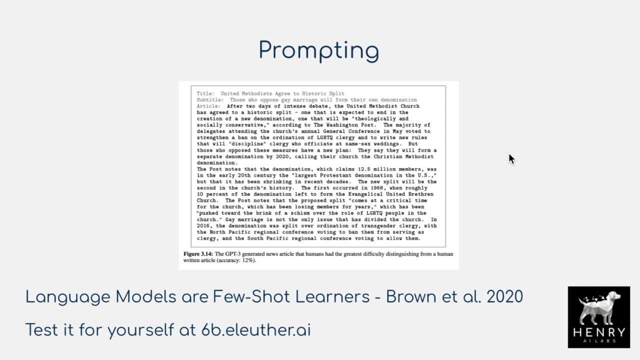 modeling. So to back up a little bit, this research is inspired by the success of prompting. Prompting, shown here in the GBT-3 paper, is where you add this context to the input to help it guide the generation. So this is exactly an example of prompting. This is where you have 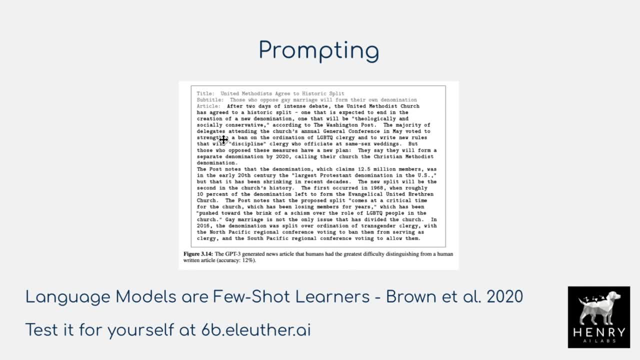 the subtitle article and you're testing the model to write an article. So prompting generally refers to adding the additional things in the input to try to guide the language model's generation, And now we're seeing a multi-modal language model with this kind of prompting. 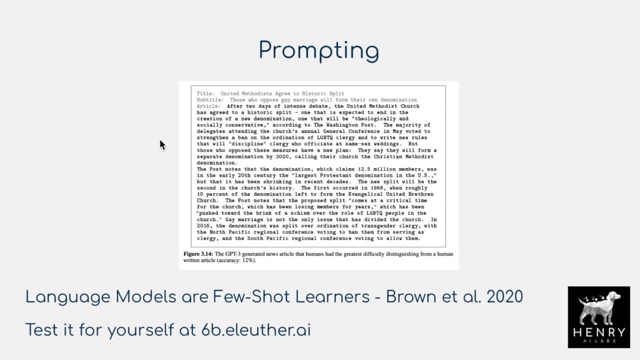 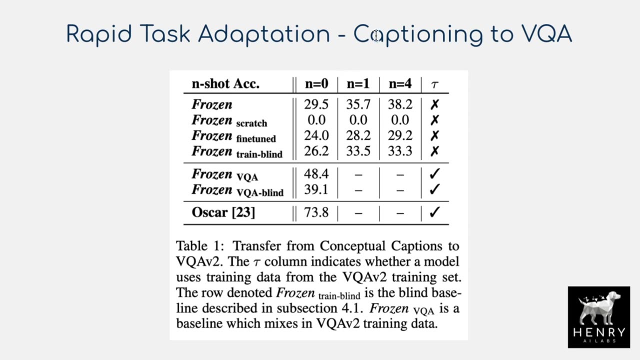 strategy where we're prompting the frozen language model, adding it to the input with these images, And I highly recommend testing out prompting for yourself in the text on the interface using this link to access the GBT-3.. The first task tested is rapid task adaptation From the pre-training of the conceptual captions. 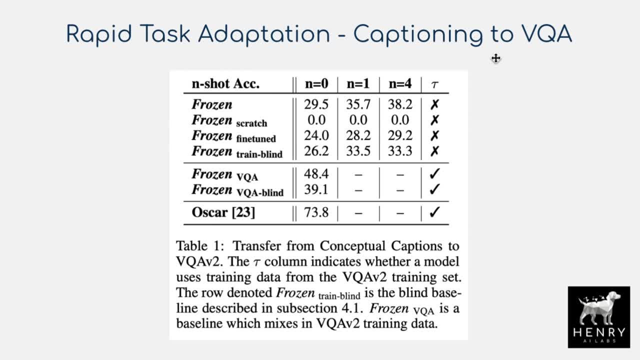 dataset where you write something like a small red boat in the water down into visual question answering like how many boats are on the water, what color is the boat, or what is the boat sitting on ideas like that. So this is the zero-shot, one-shot and four-shot transfer. 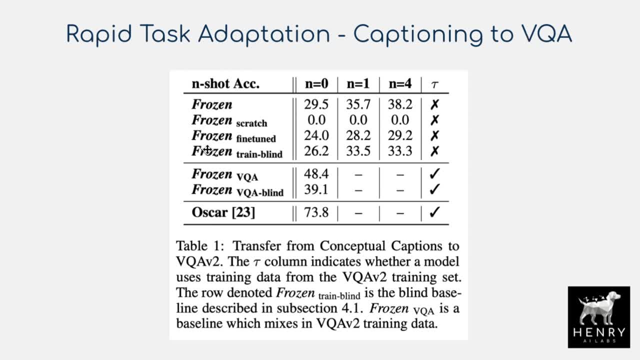 from the frozen model into visual question answering. So this is an example of task transfer in a different kind of image language task from captioning to visual question answering. And this n equals zero, n equals one, n equals four. going back to the idea of prompting, that's how many examples of the task you're. 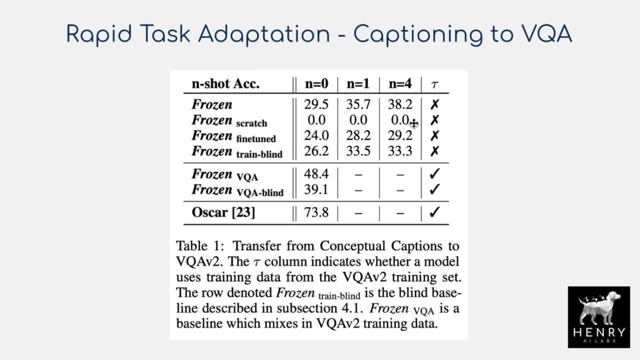 going to show in the input. So say you're asking it, what fruit is this apple? being the answer, And you add to the input: what fruit is this orange? What fruit is this banana? These kind of demonstrations are what they mean by four-shot in the context of these prompts. 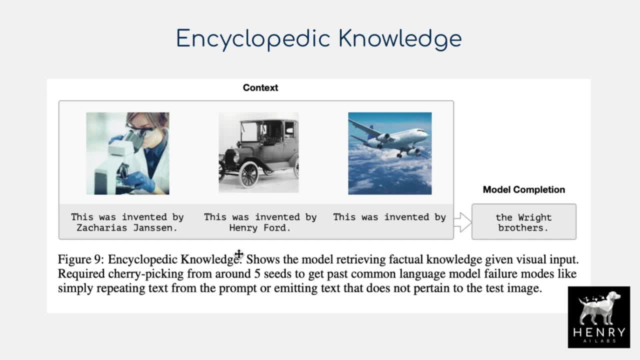 The visual question answering capability is really impressive, but the encyclopedic knowledge results are really what, in my opinion, jumps off the page with this experiment. Encyclopedic knowledge is describing being able to retrieve factual information from the frozen language model guided by the image and maybe some examples in the context as well, to help guide the generation. 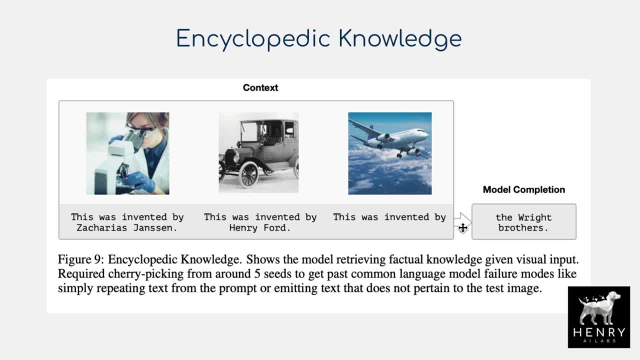 But you could just have the input of the airplane, and this was invented by and still test out. This is the idea of prompting, and then prompt tuning would be the idea of trying to find the perfect image-caption pairs that help with the knowledge retrieval that is being tested at the end. 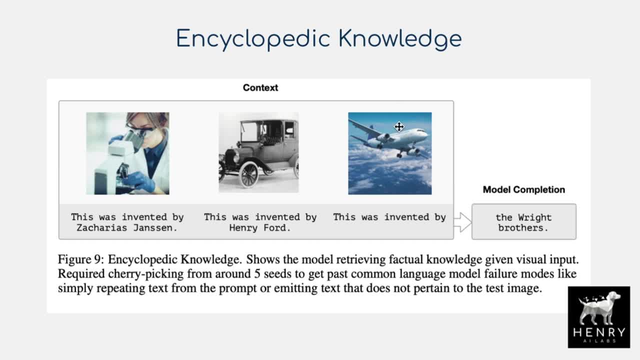 So we have these pairs: microscope car invented by, and then the airplane, and it's able to retrieve this knowledge of the Wright brothers. And again, this isn't in the pre-trained data set with the conceptual captions, because it's all hypernyms. 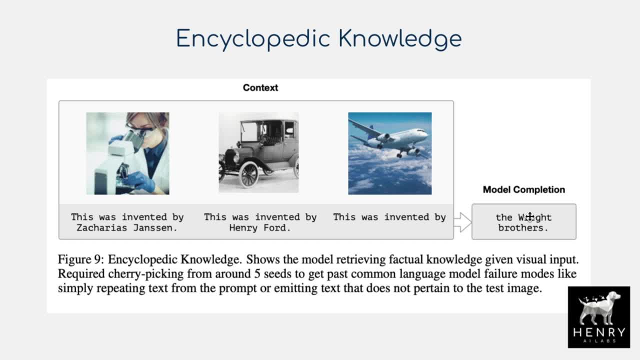 So there's no Wright brothers in the pre-training data set in the training of the visual encoder. So the language model is able to see that this is an airplane- some representation like that from the visual encoder- and then map it into the language model's representation. space reasoning capabilities. 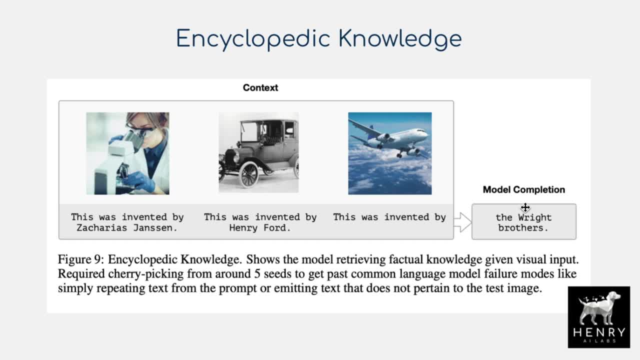 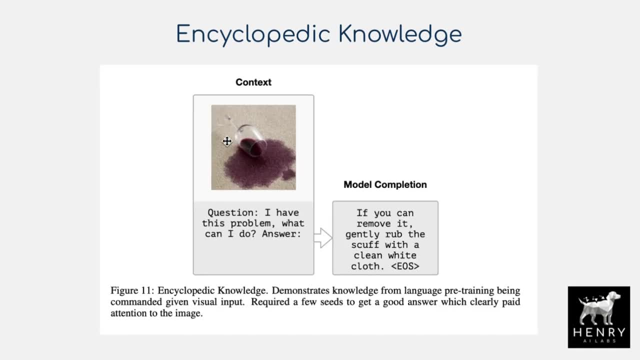 these kinds of ideas of how the language model operates And then Map it and retrieve the Wright brothers. And here are some more examples: using emojis and completing the emojis And then another example where you have a question. I have this problem. 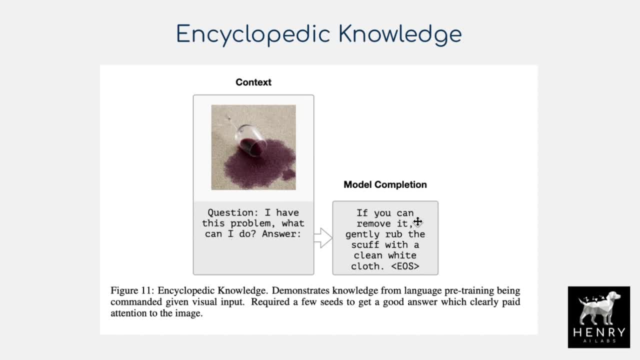 What can I do? Answer, And amazing that it's able to say: if you can remove it gently, rub the scuff with a clean white cloth from the spilled wine glass. So I think this example here is really remarkable, Noting that it hasn't been fine-tuned on visual question answering, especially with this. this isn't really how these VQA data sets are usually set up, anyways. 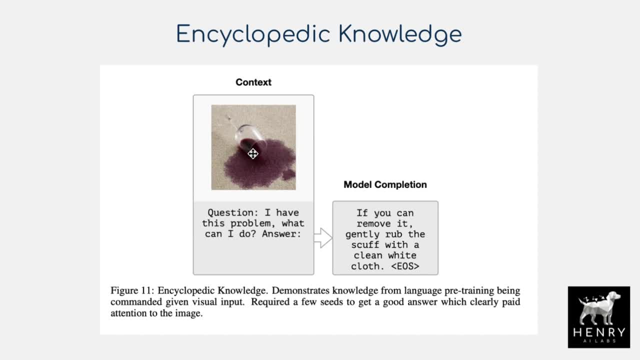 It's usually would be like: how many glasses are in the image Or what color is the stain? ideas like that It's not usually. I have this problem. What can I do about it? And then this open-ended generation answer of how you could remove a wine stain from a carpet. 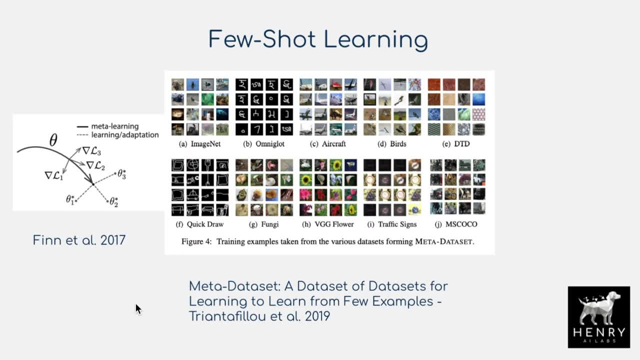 So, then, the authors are going to drill deeper into the idea of few shot learning and how it's defined in GPT three compared to, say, model agnostic meta-learning and this research on few shot learning with data sets like mini ImageNet and OmniGlot. 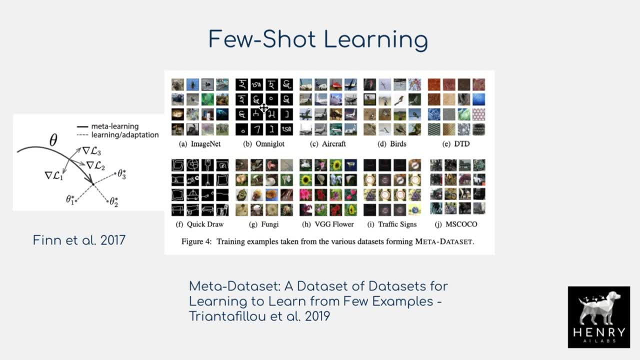 So generally we have two approaches, two families of approaches that at least I'm aware of. They're kind of the template strategies. And then The template strategies are pretty similar to the GPT three And now this frozen idea where you have this pre-trained representation that you just want to be able to quickly adapt to a downstream task through something like, say, a conditional batch normalization where you guide the parameters, or something like an efficient transfer learning with adapter layers, minimum kind of fine tuning to adapt it to, where you only say, have four examples per class to fine tune it. on some kind of idea of having this universal template that can just be adapted from the template. 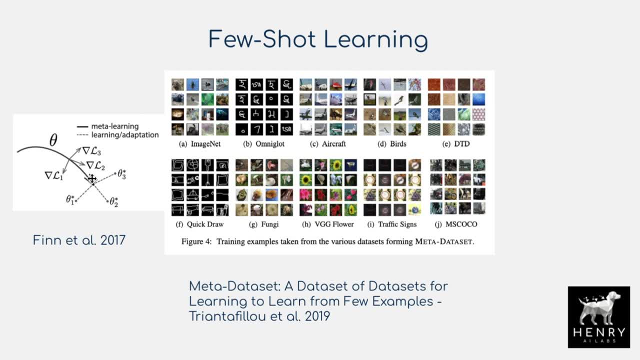 And that's kind of the idea of GPT three and frozen. and the other idea, like model agnostic meta-learning, Is to learn how to learn quickly. So you have these great, you have this outer inner loop gradient and then ideally it has some parameter space where it can learn quickly from only four labeled examples. 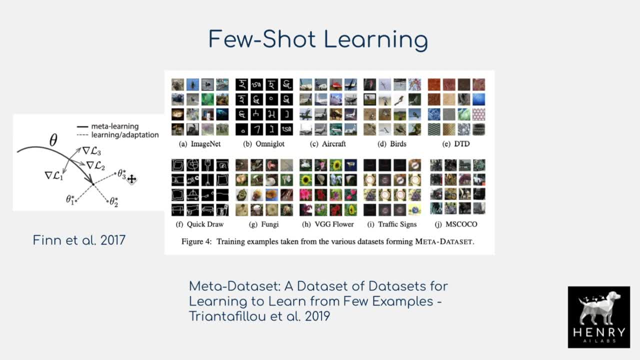 So it's kind of a different idea of learning to learn quickly and having these meta training, meta test sets for how they construct learning tasks and a bit of a more complex way of thinking about the overall scope of this problem. And you know, I don't know- have a comment on whether this will this kind of research, will how exactly it will mesh with GPT three, but it's a bigger scope of research. 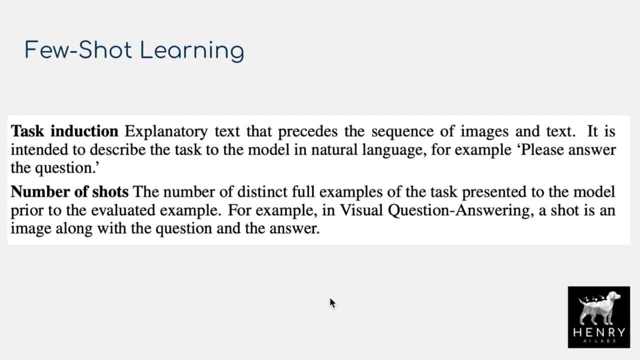 Or thinking about few shot learning. So here are some definitions about few shot learning provided in the paper. We start off with task induction and this is as shown with the spilled wine glass example of. please answer this question or I have a question. what should I do about this? 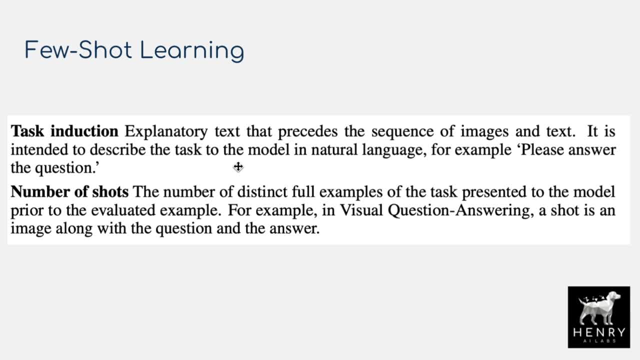 This kind of idea of inferring the task is being applied. This kind of reminds me of the T5 text to text transfer transformer paper. When I first read that paper I thought that the way it was doing it was by having natural language descriptions of the task. 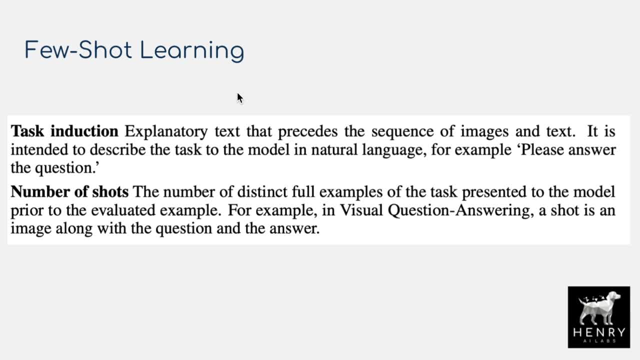 I'm not sure if they one hot encode the different tasks or whether it really is natural language descriptions. But imagine Just having you unify all these tasks into the text framework. So it's a text classification, you know, colon, and then the input, natural language inference, the inputs, question answering the inputs, that kind of way of giving the model the sense of what task it's supposed to perform. 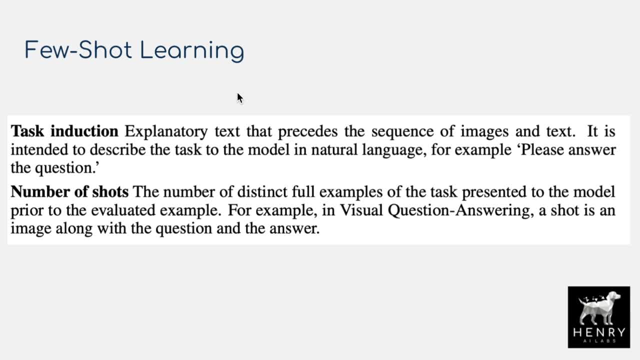 Whereas language modeling- there's a paper in the ACL catalog titled something like language modeling is multitask learning- because in language modeling you do have to kind of infer these different tasks in a way, in the way that this mass prompt requires you to do it. 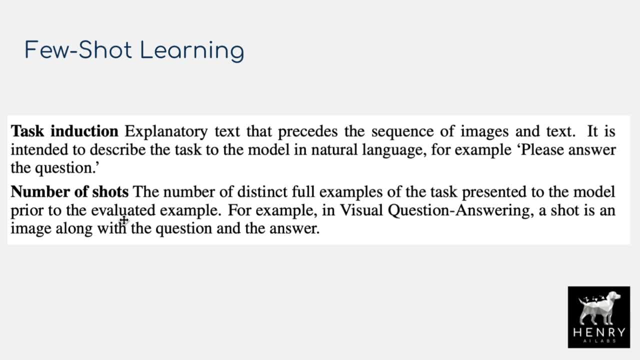 In order to you know, complete the correctly masked out token. So the next thing, common thing, this idea of the number of shots. when you say few shot, you're describing how many examples are given. So one shot means you have one example, two shots, three shots, so on. 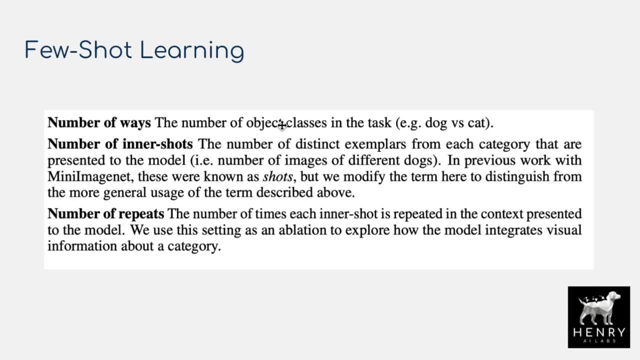 So. so, drilling into this further, they define the number of ways, which are the number of object classes. in the task of, say, CIFAR 10 would have 10 ways, 10 object classes for classification. Number of inner shots is again this idea of shots, but maybe more specific to the inner category when you're sampling the shots for 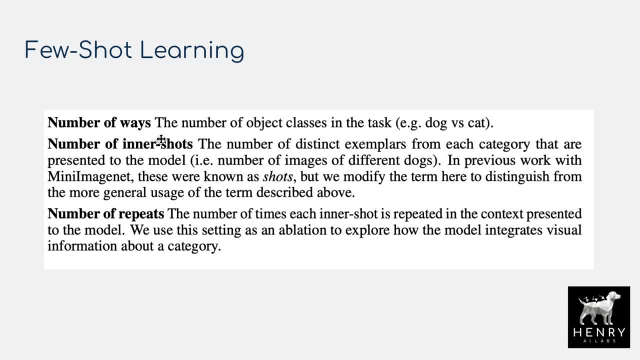 So I think what this means is that the overall scope of this could have 10 ways, so 10 classes, and then it only sees three shots, So dog, cat, airplane or some idea like that is what I think they're trying to communicate with: the distinction between the overall cardinality of possible class labels and then what's seen in the few shot demonstration context. 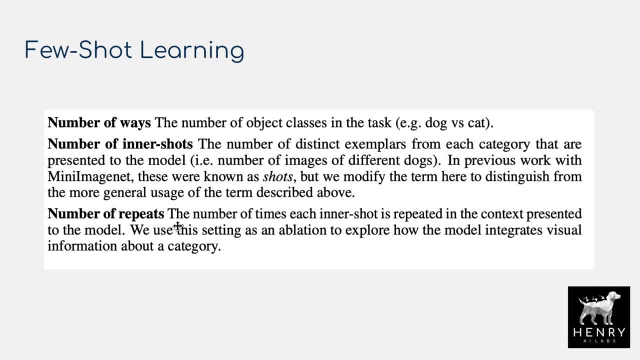 And then the number of repeats seems to be how many times you repeat the same class. So how many dogs, how many cats? this kind of idea of further breaking down the distributions and the inputs for a few shot learning- And I'm not exactly sure if that's what they mean by this, but at least that's how I interpreted it and hopefully that's useful for you. 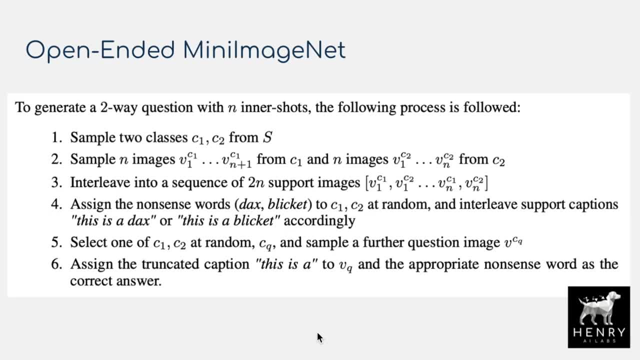 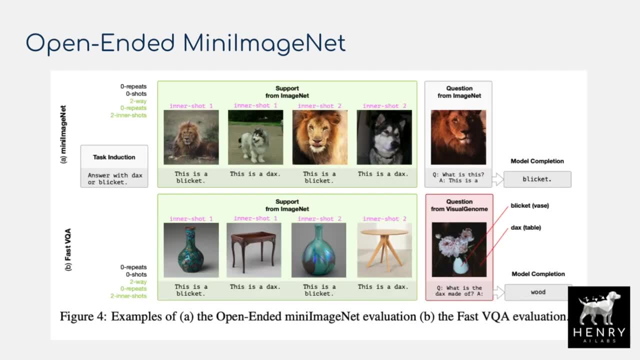 So next up, we're testing this idea of visual concept binding and constructing a new data set titled Open Ended Mini ImageNet. So the way this works is we're generating a two way question with an inner shot. So to further, here's the illustration of the idea, and inner shots means, for this case, two lions, two dogs. 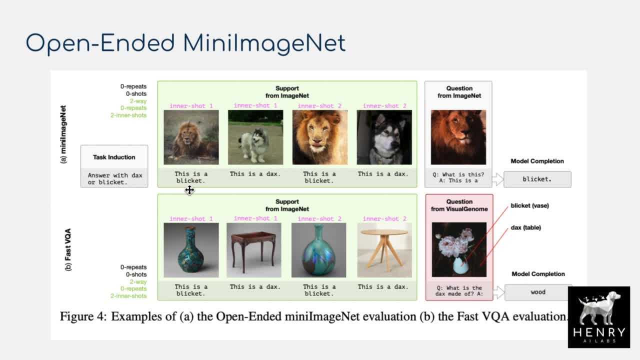 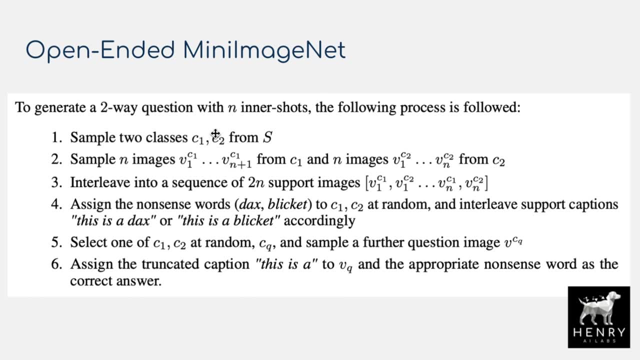 And then the fast concept binding means we're going to reassign lion to be blicket and the wolf is dax. So this is the template for constructing the data set. You select two Classes, as a lion, wolf, from the S, which is the number of object categories. sample, in this case: two images of the lion, two images of the wolf, and then you interleave the sequence that you have: a wolf, lion, wolf, lion, wolf. 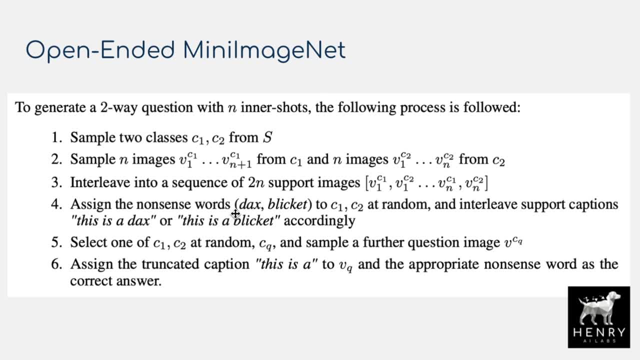 Then you reassign the lion wolf to nonsense words: dax, blicket, at random, with respect to which one you sampled. Then you sample the question image, So you append the prompt- This is a, and then the nonsense word, And then you have as the 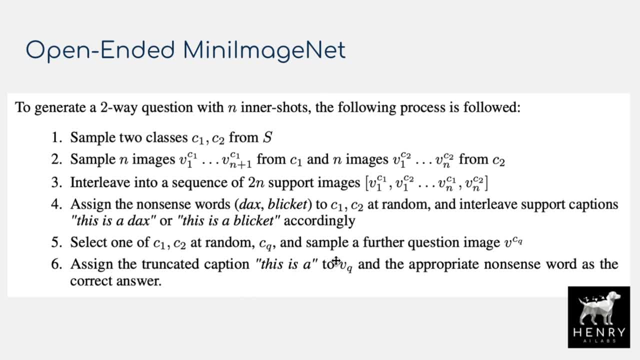 The inference uh, the truncated caption. This is a to the uh VQ. VQ is the question template, So just question colon or however you want to ask the question. This is here. I have a question for you. whatever you can imagine as a natural language description of the question. 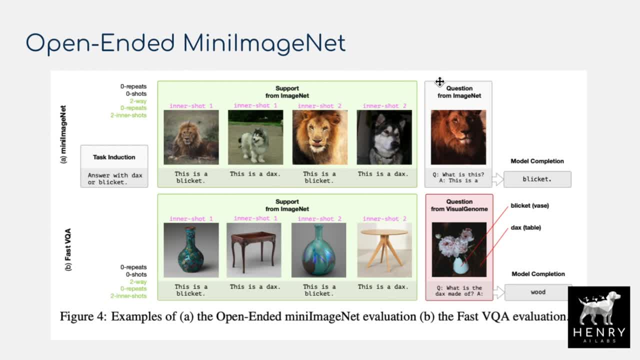 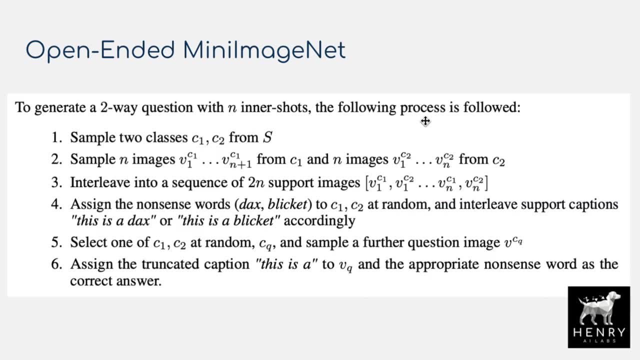 And that's used to form this mini image net data set And you can have many ways of sampling. You can sample a thousand different of these prompts. given the data set where as input you have the set of images and then the uh object classes, this paper is presenting a really interesting 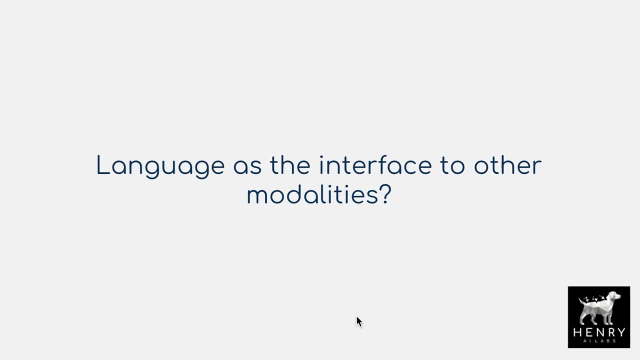 Idea that language is a good interface for combining other modalities in this multimodal learning, And the language layer may be the most important layer in these multimodal representations And it seems. it seems to make sense because the language models are trained on so much knowledge intensive data that it's really different from most of these other tasks. images or, uh, videos, maybe videos, but audio, these kinds of data sets. 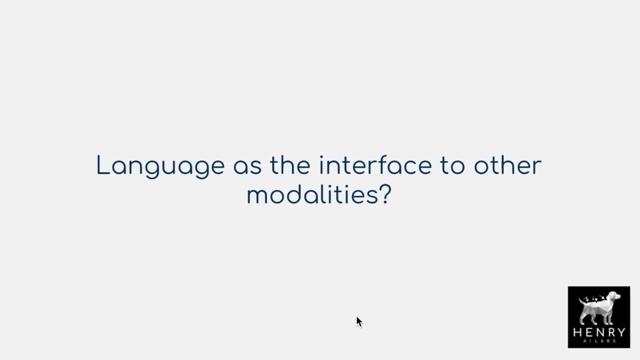 I don't think they convey as much information as these. you know, like hundreds of gigabytes of text, data scraped from Wikipedia, Books and all these ideas that will describe these visual concepts somewhere in them, And maybe they just need a little bit of grounding from the visual encoder, audio encoder, video encoder, as shown in this data set or other modalities. 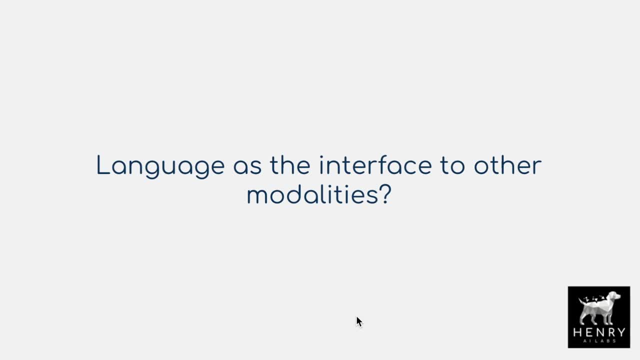 We can imagine like, uh, touch, as you have this encoding of, say, robot sensors or LIDAR sensors or all these different other kinds of ideas. So I think it's interesting thing about language is the interface, these other modalities, And clearly this experiment has shown that this strategy works to some degree, and they do note that this isn't the state of the art for visual question answering or any of these other vision. 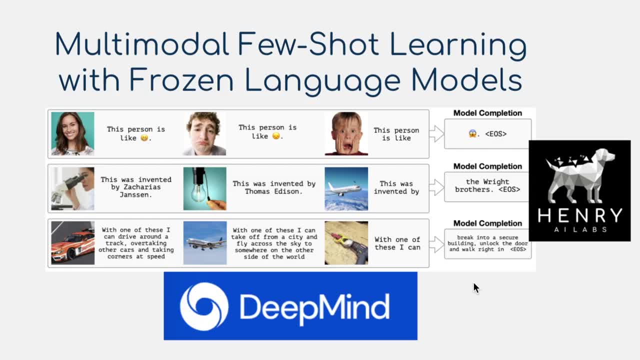 language tasks, but the fact that this works at all, I think, is pretty remarkable. Thank you so much for watching this quick overview of multimodal few shot learning with frozen language models, One of the most interesting papers that have come out recently, with a really surprising result of being able to freeze the language model, train a vision encoder and then 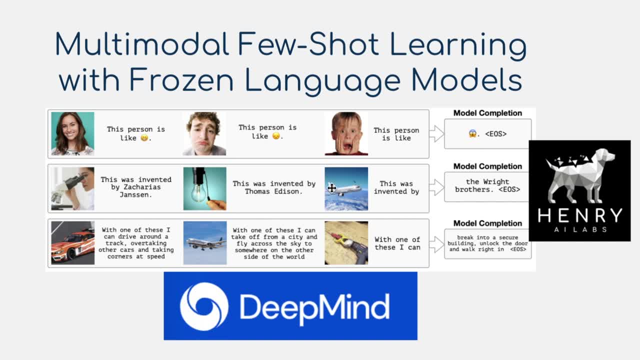 perform these few shot learning tasks with visual inputs, where it does things like uh adaptation from captioning to visual question answering, uh, this encyclopedic knowledge retention, and then this idea of uh quickly- this is not shown in this image, but this idea of quickly being able to buy new concepts, like